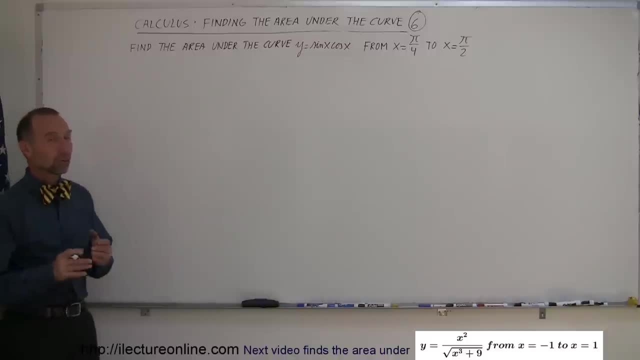 Our next example of how to find the Erring-Nieder curve is actually a specially chosen example to see how you work with the limits where we have to use the method of substitution to integrate the function. The function here is the sine of x times the cosine of x. The limits are from pi over. 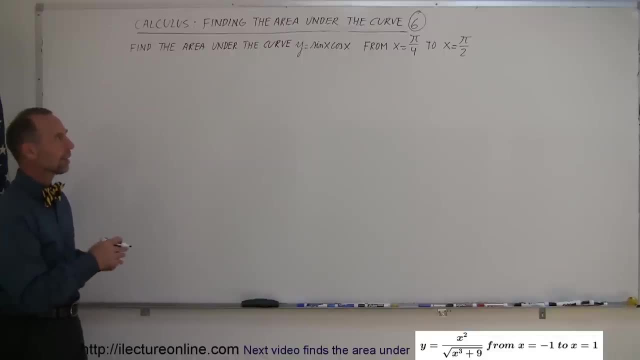 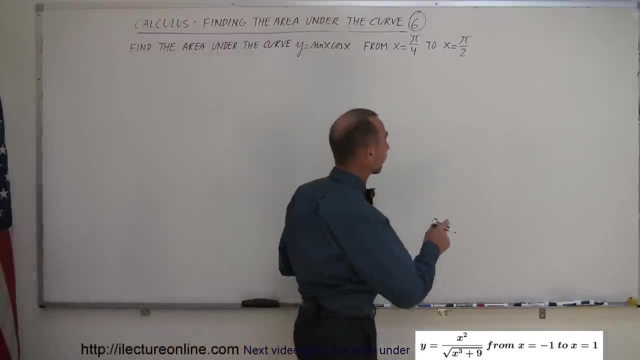 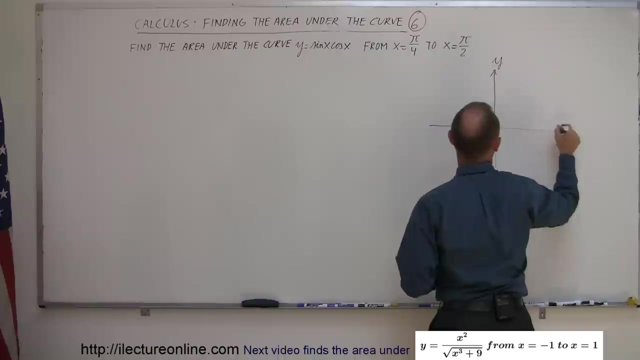 4 to pi over half. So how do you integrate that and how do you find the limits? and how do you find the Erring-Nieder curve? Well, let's try to graph the function. So, first of all, it's a product of two functions. so we have the y-axis, we have the x-axis. First let's graph the sine of. 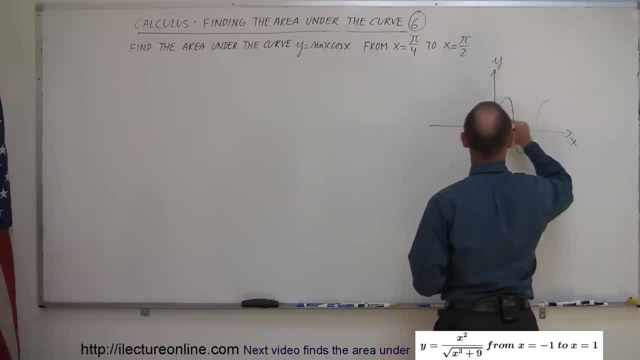 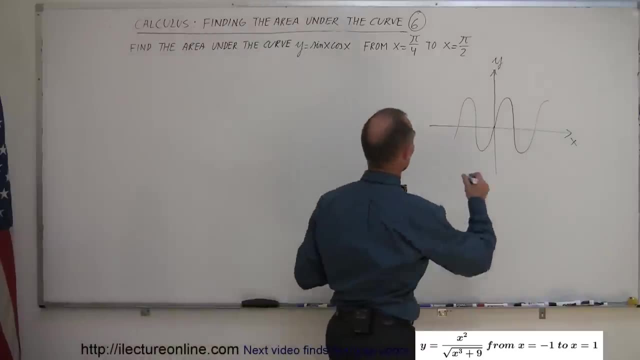 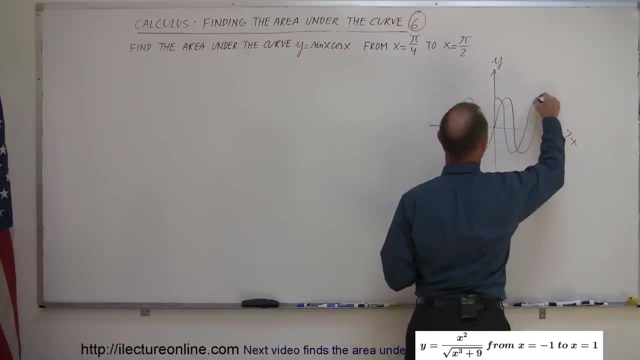 x. The sine of x looks like this. and now let's grab the cosine of x. I'm going to use a different color for that. The cosine of x starts like this and goes down like that, comes up and goes like this and like that, And now notice that we're trying to find the area underneath the cosine. 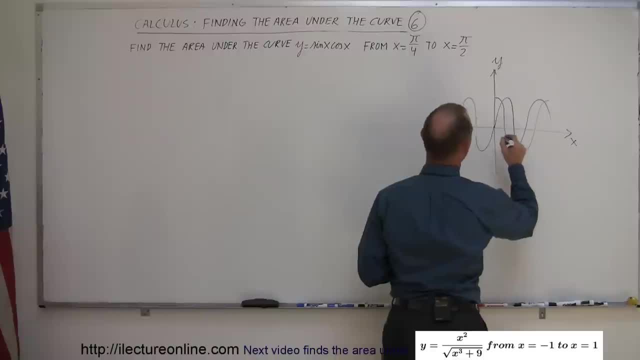 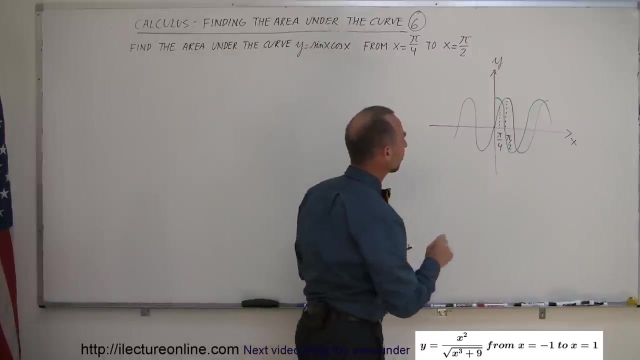 curve from pi over 4, which is from about right about here- this is pi over 4- to pi over 2, which is right up here- pi over 2. maybe I should have made it a little bit wider made, it might have made it easier to see. but at least what we can see is that both functions, both the sine of x. 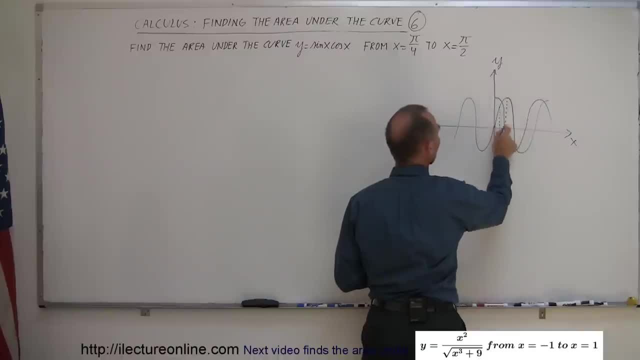 and the cosine of x are either 0 or positive between the values of pi over 4 and pi over 2, so do you know that the product between the two will also be positive, and so you can see that the product of the two will probably be something that looks like like this. so the product looks like. 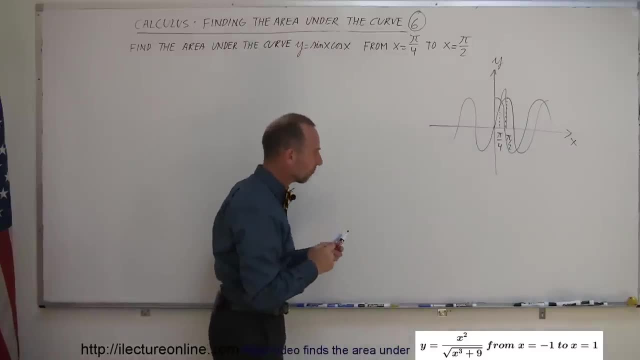 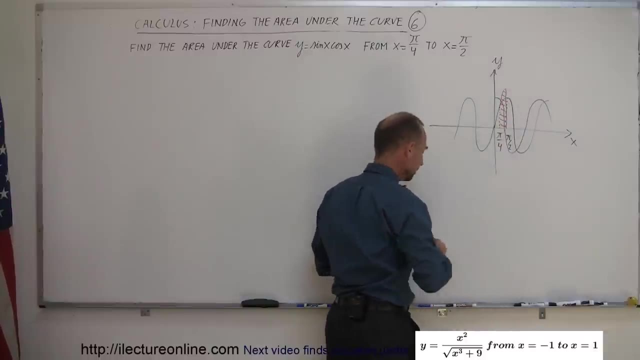 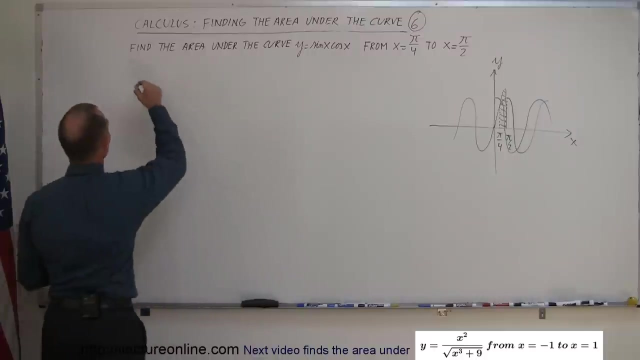 maybe something like that. I'm just guessing, but you know, not that far off, and we're trying to find the area underneath this curve, right here, like so okay, that gives us at least a visual picture of what we're trying to do now mechanically. how do we get through this problem? well, first of 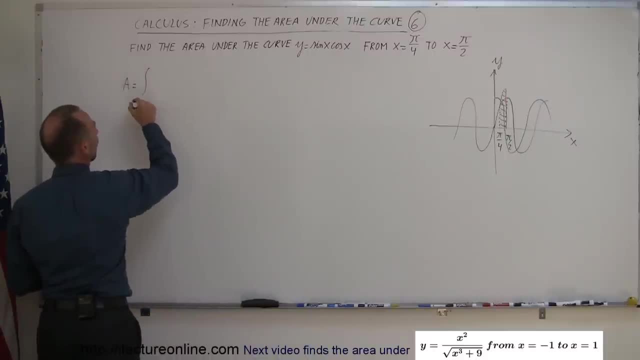 all, we can see that the area is equal to the integral from x equals pi over 4 to x equals pi over 2, from for the function sine of x, cosine of x times dx. all right, how do you integrate that? well, it turns out that the 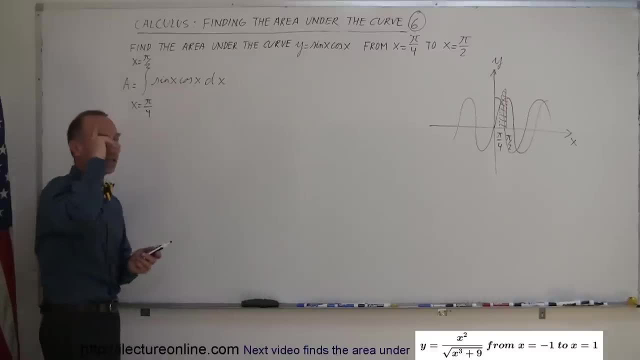 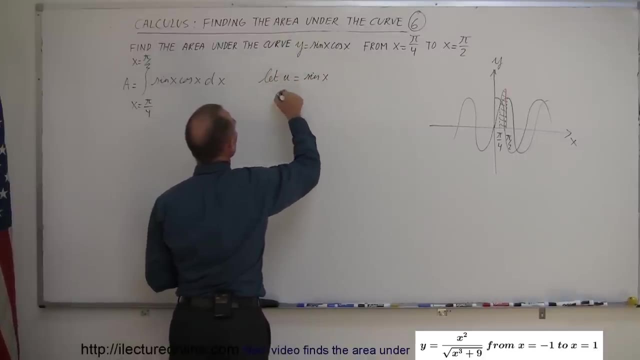 cosine of x is the derivative of the sine of x, which gives me an idea. I say: okay, that means if we let u equal the sine of x, then du, dx is equal to the cosine of x and therefore du is equal to the cosine of x- dx, which means I can. 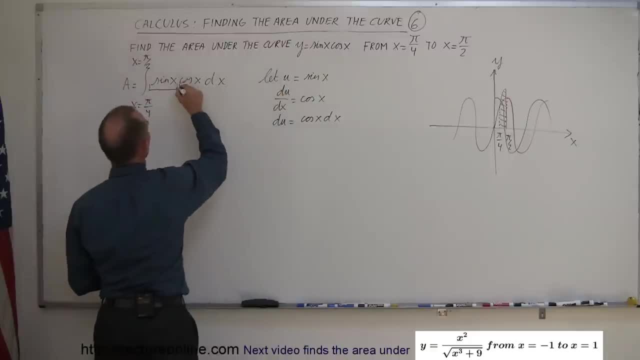 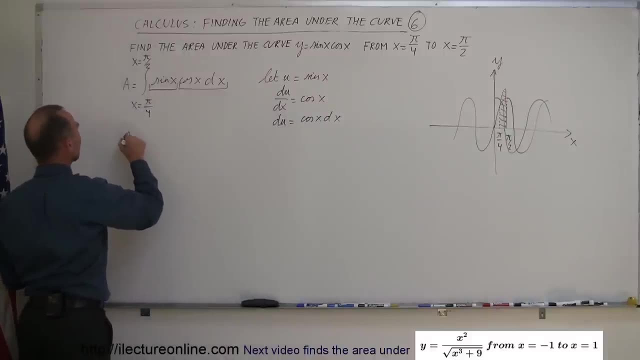 replace the sine of x by u and I can replace the cosine of x dx by du. if I do that, I get the following integral: a is equal to the integral of u times du, with the limits of x equals pi over 4 to x plus phi over 4, and y equals thepee over bi over 4 and z equal to x minus z equals 2 pi over 4. 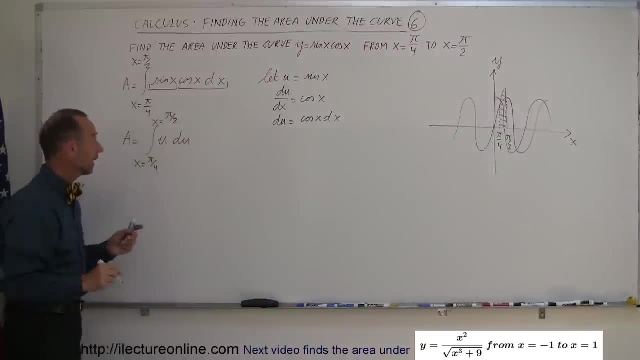 x equals pi over 2.. Now notice that I did write the limits are: x equals pi over 4 to x equals pi over 2, even though the variable I'm using in my integral are u's. So once we do the integral we cannot just blindly plug in the limits because they're not the right limits. So just to see what: 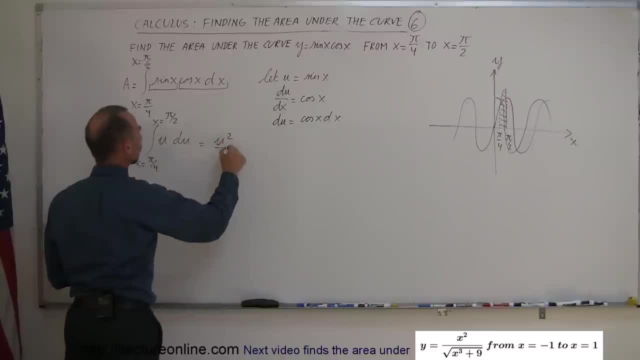 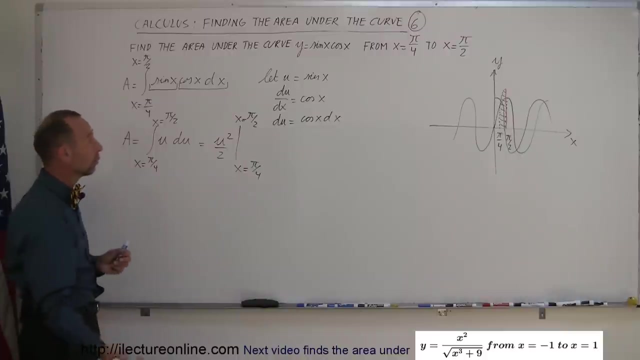 we do in just a moment. So the integral of this is u squared over 2 from an evaluated, from x equals pi over 4 to x equals pi over 2.. Now we can't plug in the limits because the limit variables do not match the variable I have here. So what I have to do now is resubstitute back in, but u. 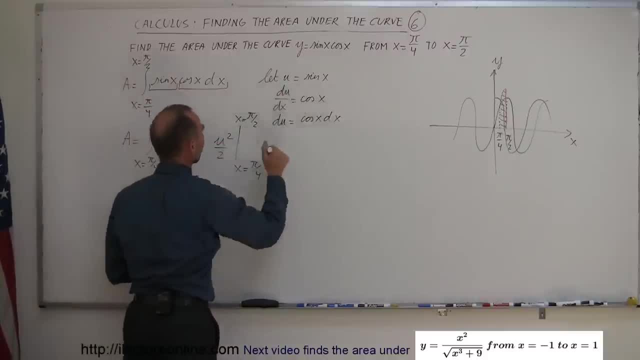 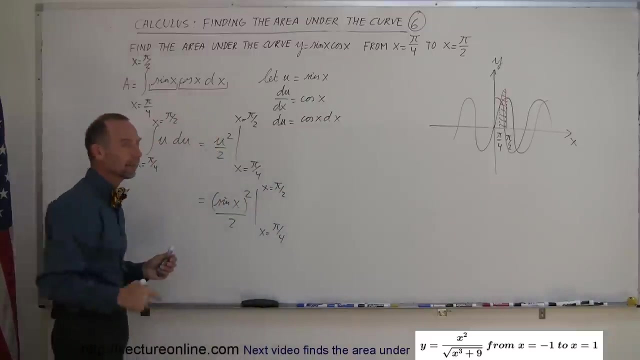 is equal to and u is equal to the sine of x. So this can now be written as: the sine of x squared divided by 2, and evaluated from x equals pi over 4 to x equals pi over 2.. Now I'm ready to plug in my integral. 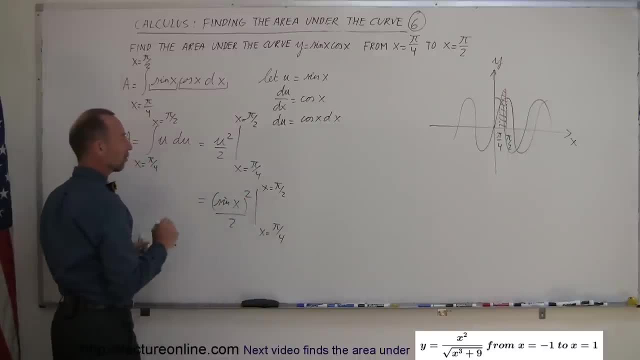 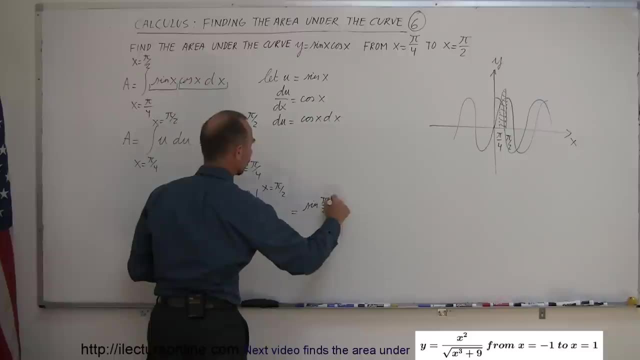 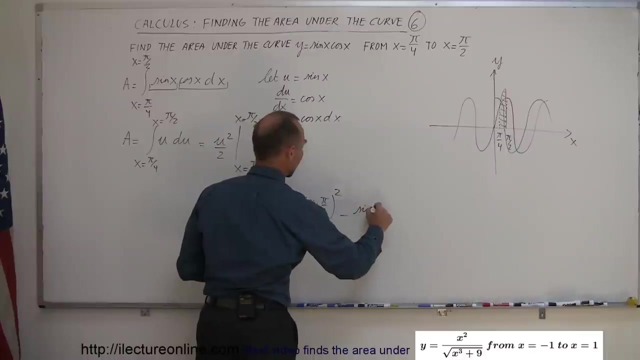 limits, because now the variables here match the variables on my limits. Okay, so this is equal to: when plug in the upper limit, we get the sine of pi over 2 squared over 2 minus. when plug in the lower limit, that would be the sine of pi over 4 squared divided by 2.. All right, now what is the? 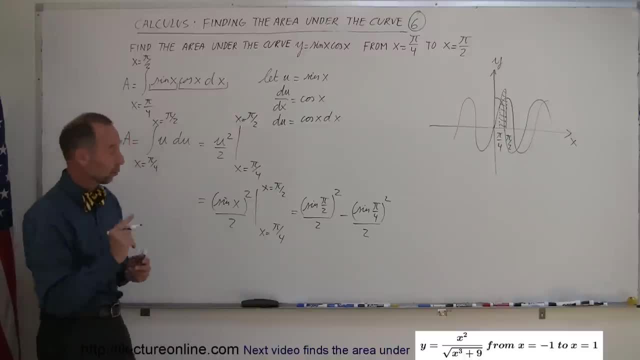 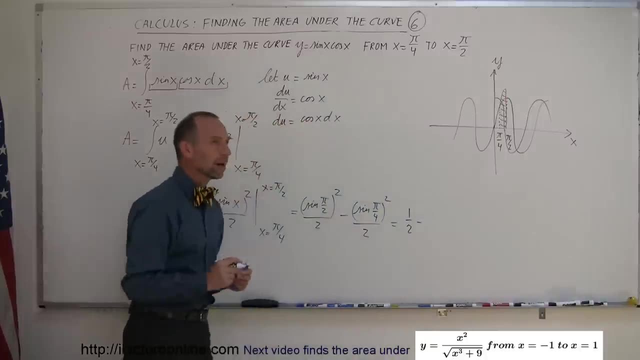 sine of pi over 2?? Pi over 2 is 90 degrees. The sine of 90 degrees is 1.. So this would be 1 squared over 2.. So this would be 1 squared over 2, or 1 half minus the sine of pi over 4, that's 45 degrees, which is.